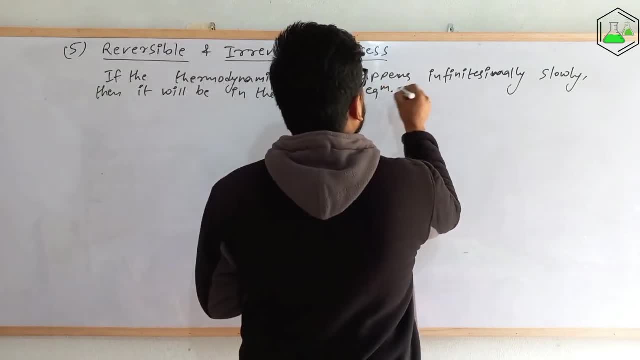 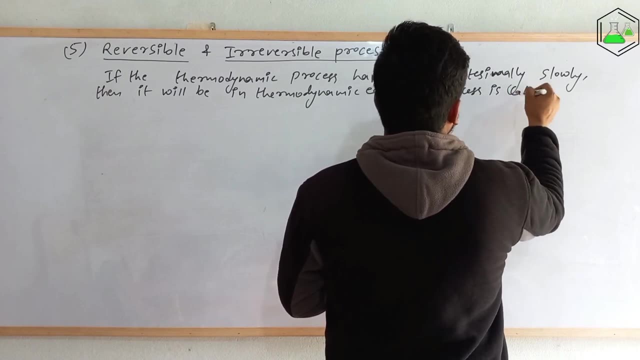 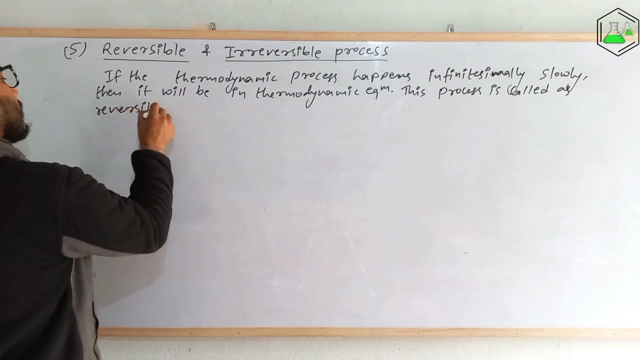 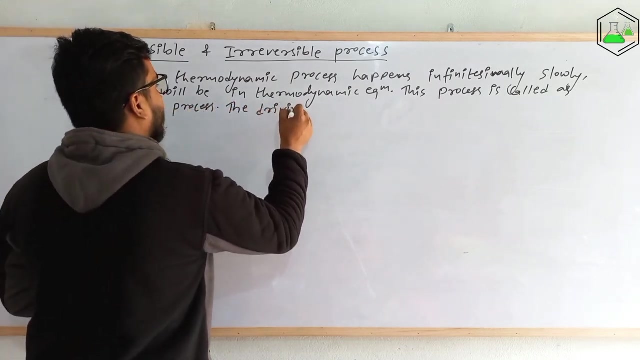 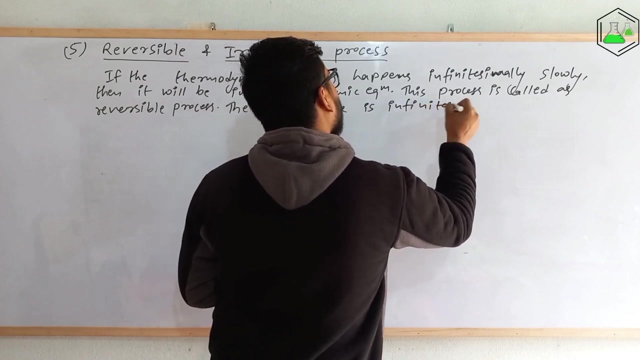 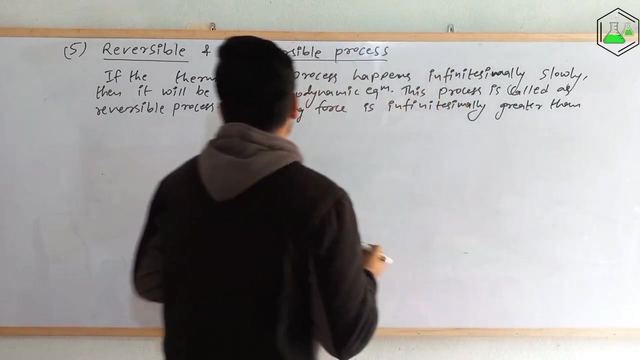 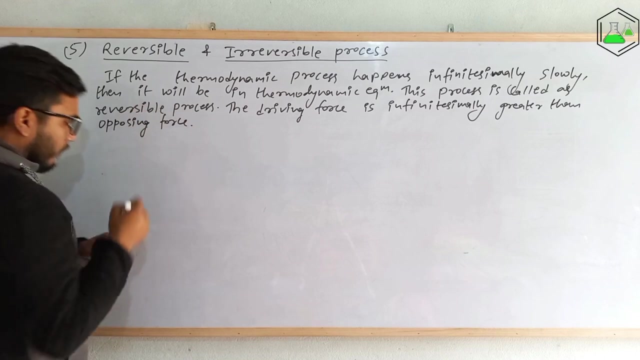 equilibrium. This condition or this process is called, is called as equilibrium, reversible process. reversible process: reversible process: the driving force, the driving force is infinite, is only greater than greater than opposing force. opposing force, that is, the driving force will be slightly greater than the opposing force. then that type of system will be in thermodynamic equilibrium. all. 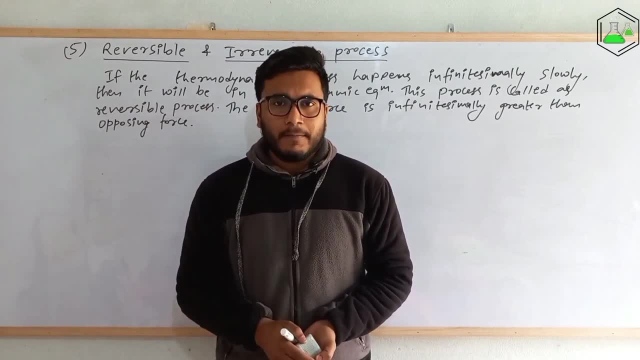 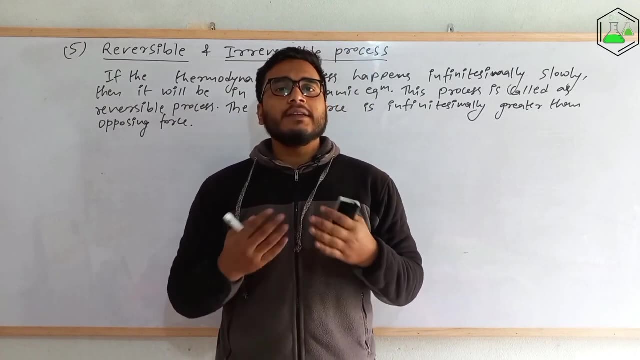 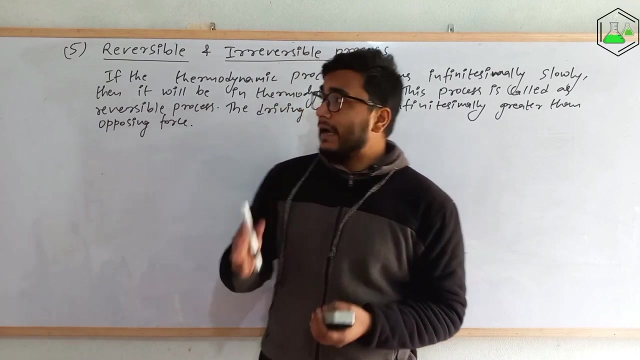 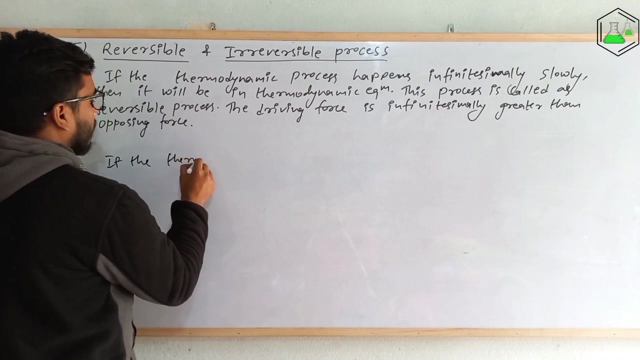 the time and that is called reversible process. but irreversible process means sudden change. okay, if the system is, if the thermodynamic process is happening suddenly, then obviously that will not be in thermodynamic equilibrium and that type of process is called irreversible process. so if, if the thermodynamic process, if the thermodynamic process, 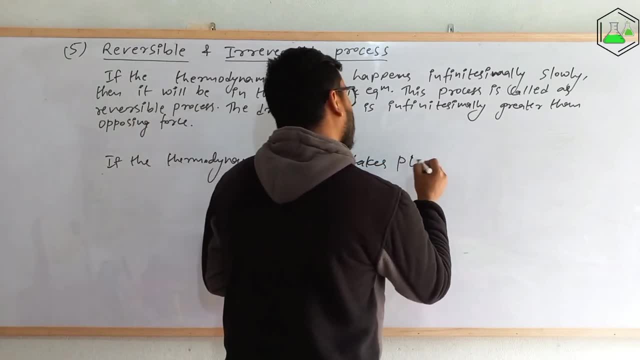 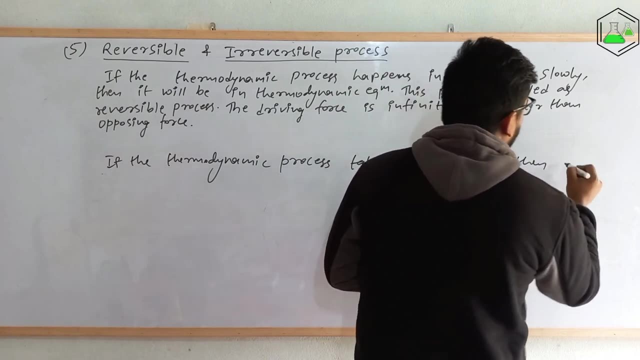 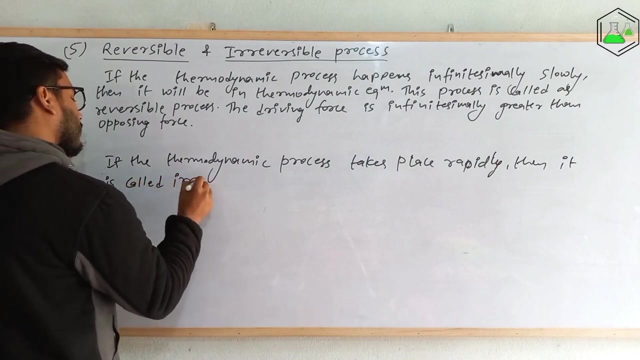 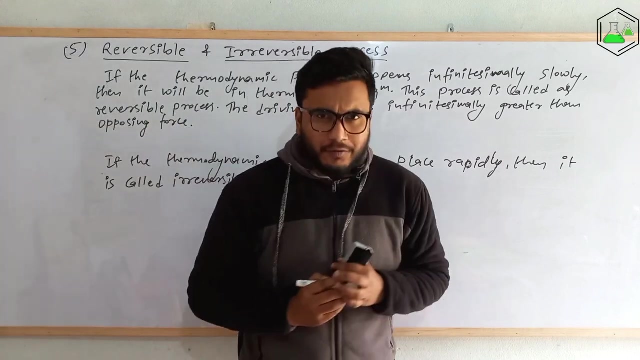 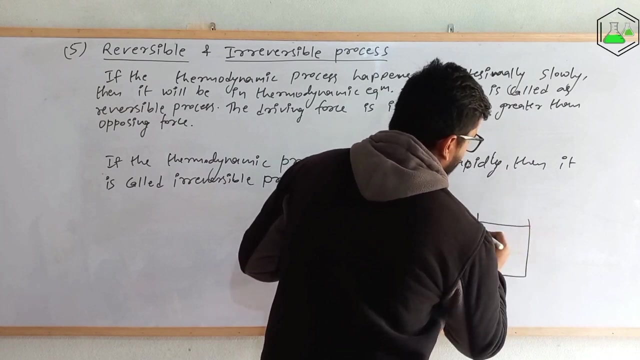 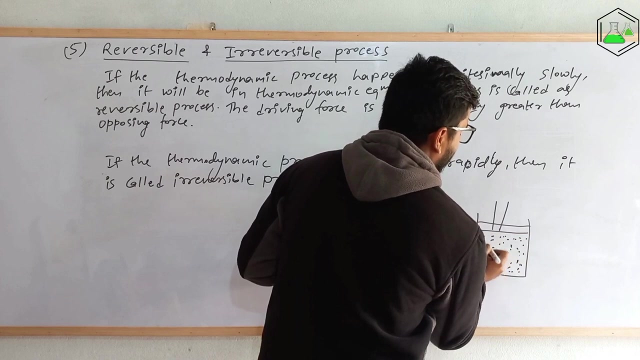 takes place, takes place rapidly, takes place rapidly then. then it is called irreversible process. we reversible process, irreversible process, but confused. let me explain this with a simple diagram. suppose there is a cylinder in which there is gas and this is a weightless and frictionless piston. obviously, this does not exist in real life, but still, let's consider. this is the 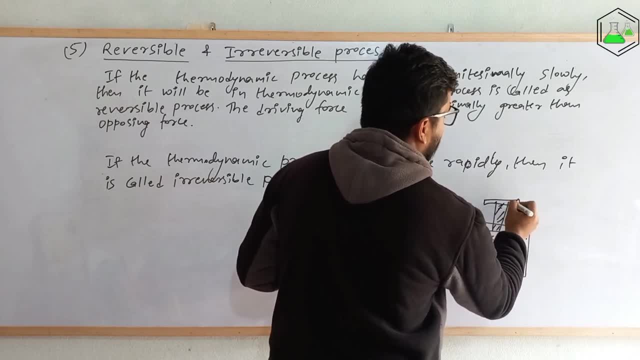 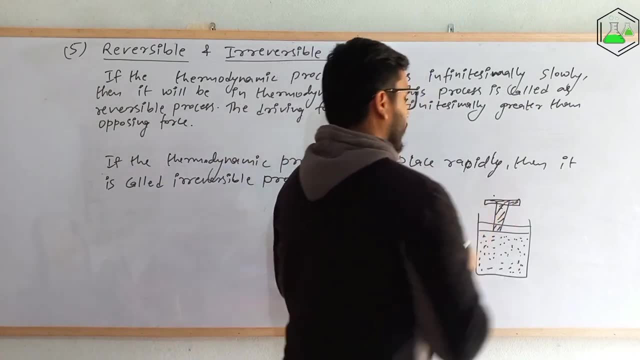 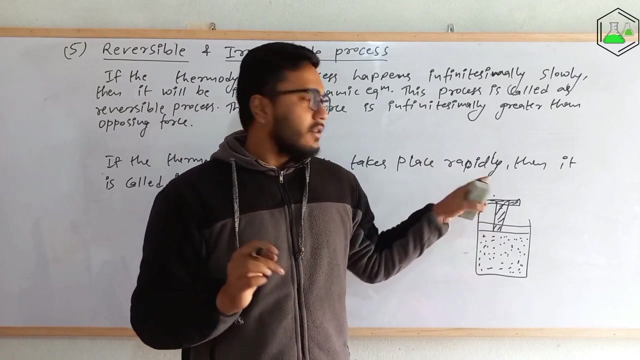 weightless and frictionless piston. okay, now over it. let's drop one, only one sand, one sand. we drop it. what will happen? the piston might go little bit inside and it happens so slow that the thermodynamic equilibrium will be managed over there, will still be over there. let's drop another.